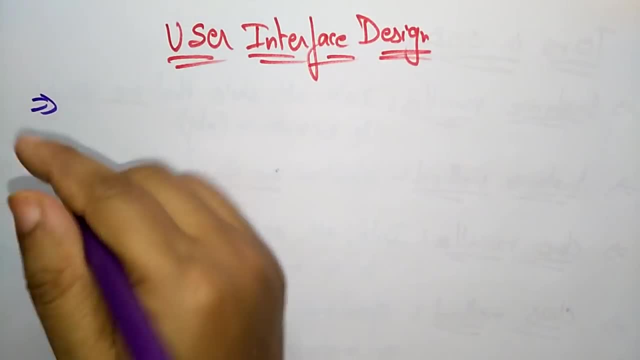 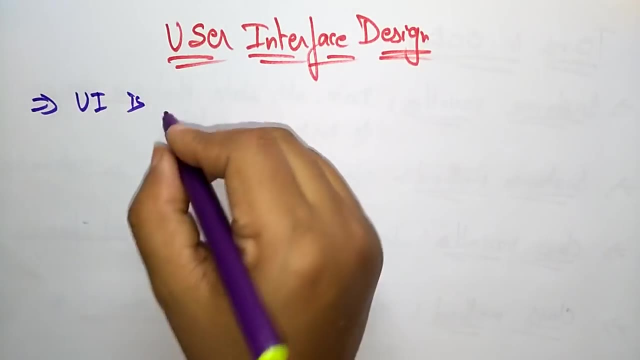 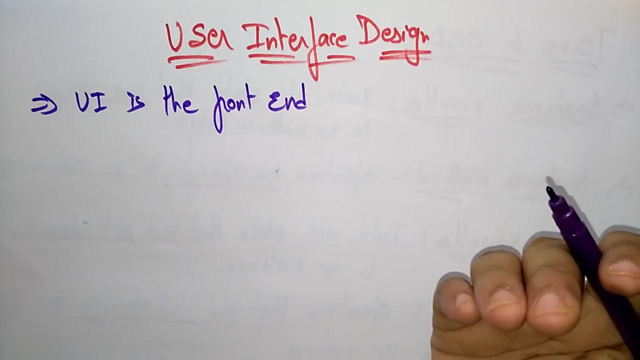 So the user interface is first, it is a front end. The user interface is. so I'm writing UI as a user interface. User interface is the front end application. We call it as a front end application because we are accessing that page, So that is present in front of us. So that's why we call it as a front end application. 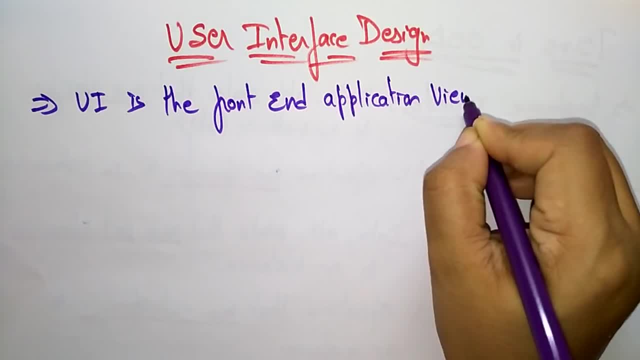 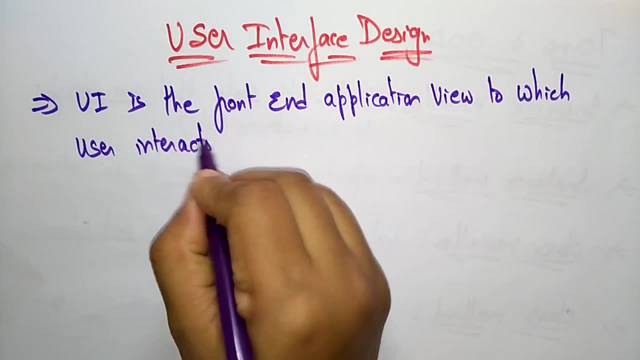 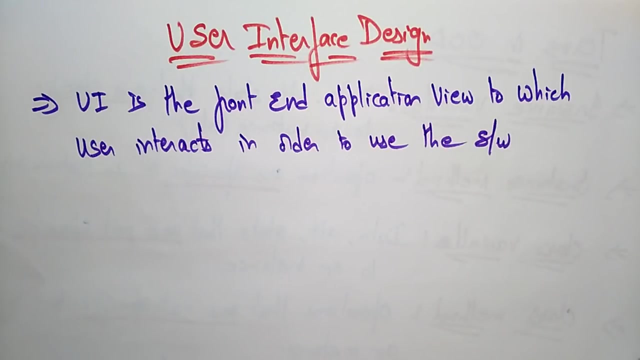 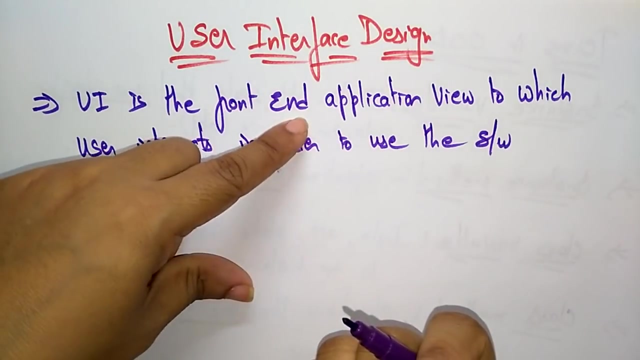 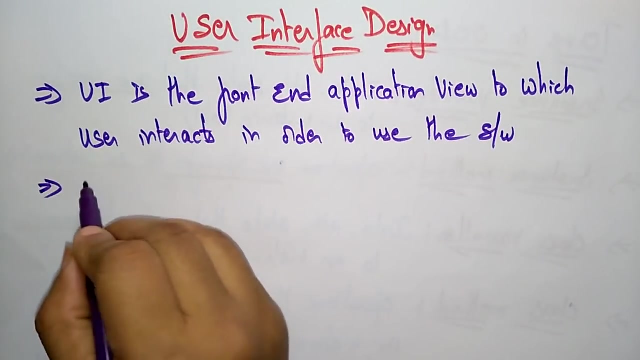 It is a front end application view to which user interacts in order to use the software. So the user wants to use the software. So with the help of this user interface applications. So the user interface application is a front end application view to which the user interacts in order to use the software. So here in the user interface design, user can manipulate. 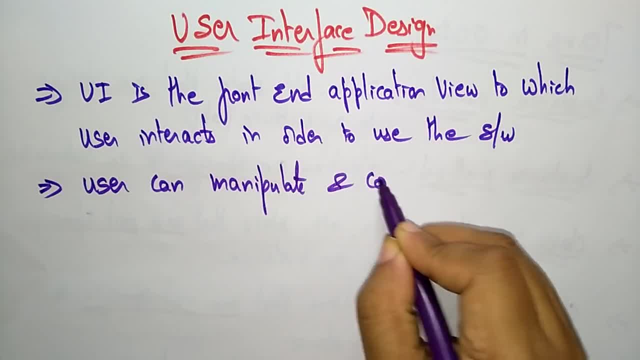 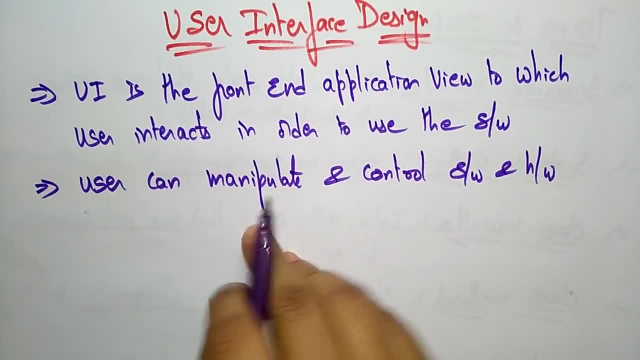 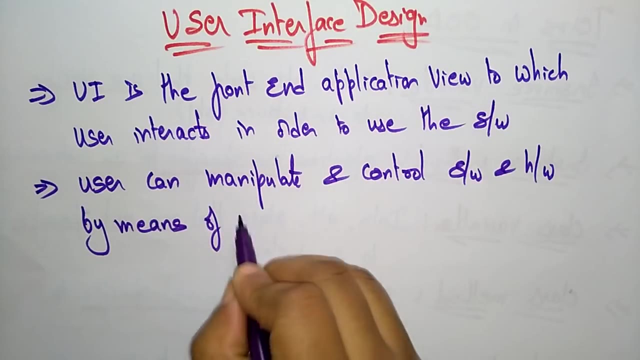 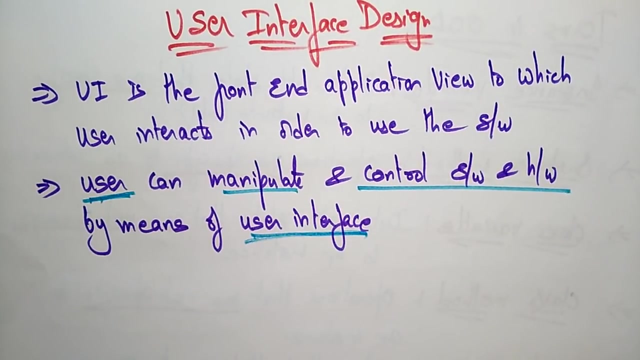 manipulate and control software and hardware. so the user can have the permissions to manipulate and control the software as well as the hardware by means of, by means of user interface. so, with the help of the user interface, only this user, that user, can manipulate and control hardware as well as the software, with the help of this user interface. so let us take one example. 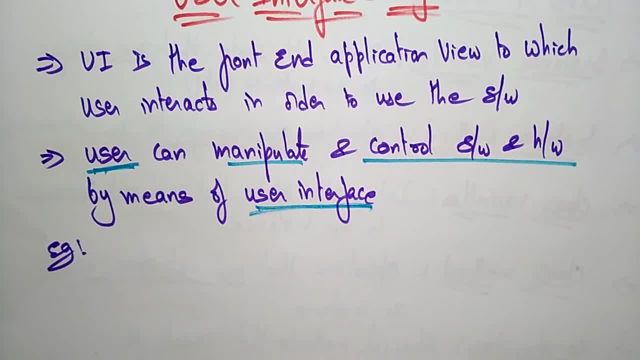 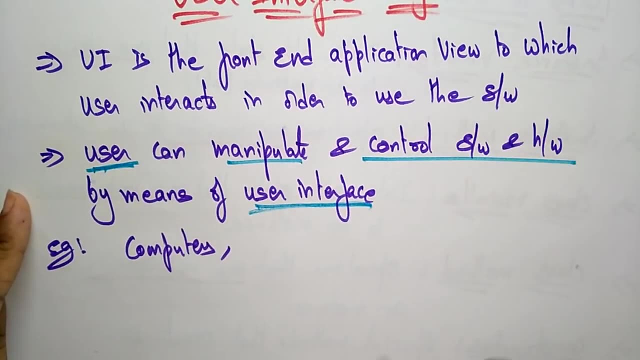 so in this example, suppose today, whatever user interface we are founding is is found at most every place, like where, in digital technologies that exist, so like right from computers, in the computers we are having the user interface, so which you are seeing on the screen, so the windows desktop, whatever you open, that is an user interface. 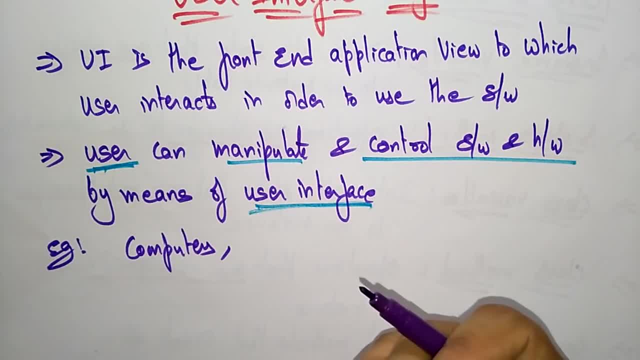 okay, so that's a. if you want to manipulate and control any software and the hardware in your system, you need some user interface, uh, this device. so with the help of this user interface, you are going to manipulate and control all the softwares that are present in your system. 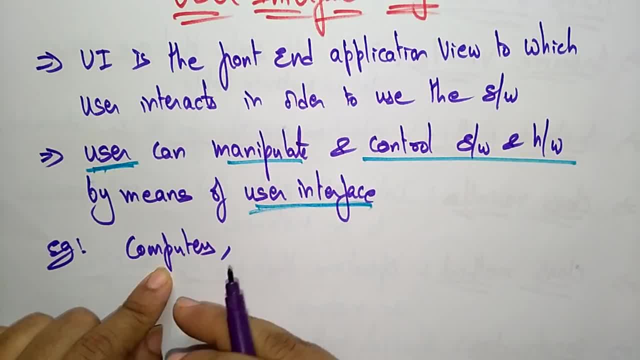 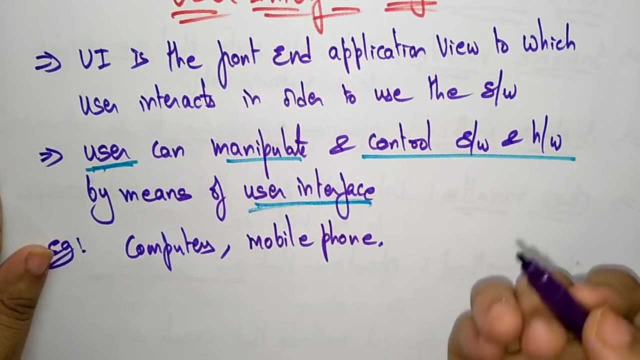 as well as the hardwares. so, just like a computer, a computer is is one of the user interface. design means it. uh, a user interface is found in computers in the same way in the mobile phones. okay, so in the mobile phones you are having, the user interface means whatever you are seeing on. 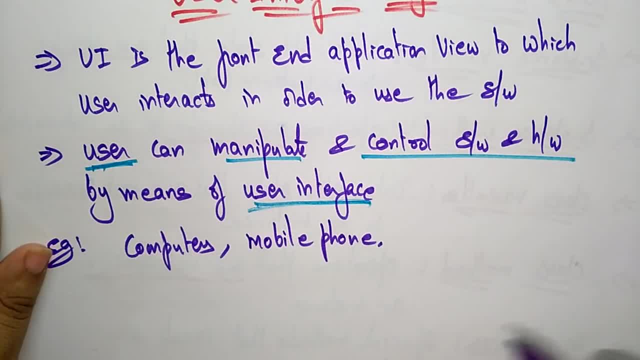 this mobile phone that is a user in user uh view. it is a front end, which is an applicati user interface, which is a front end application view. so that will be provided in mobile phones in the same way, in the cars or in airplanes, even in music players, everything you can find. 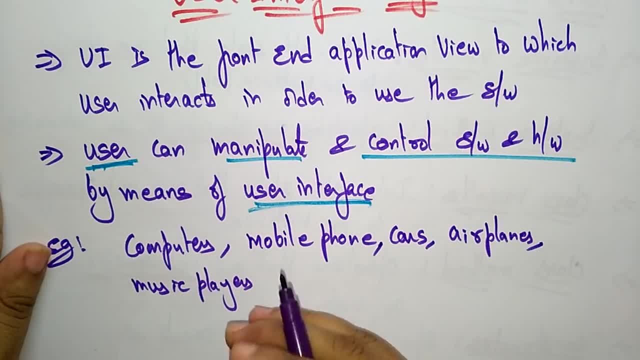 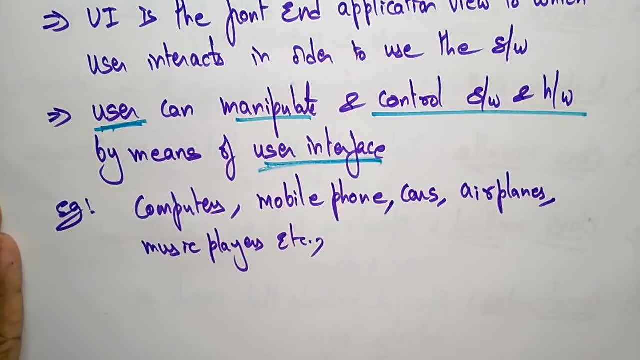 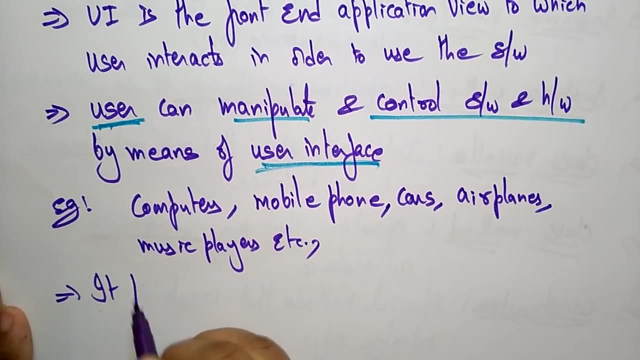 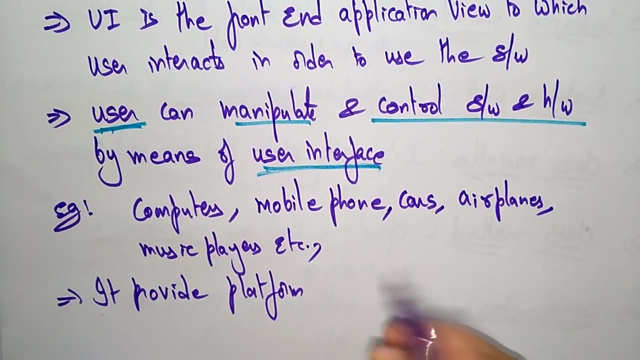 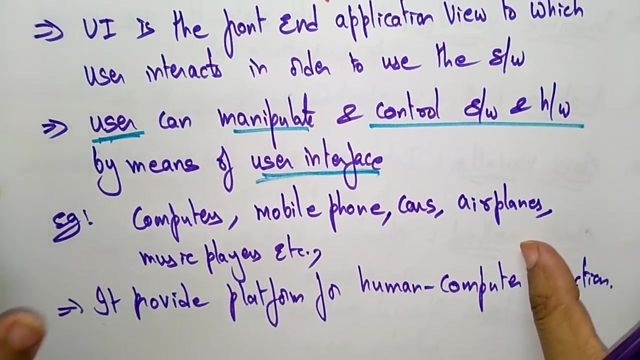 every digital technology you can find the user interface. so this is something just to interface, etc. okay, so this user interface provides fundamental platform for human computer interaction. it provide platform. this user interface design provides a platform for human interaction and it is also a part of a software, so this user interface can be graphically text. 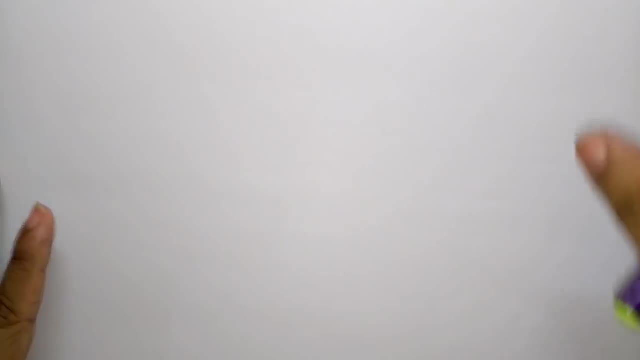 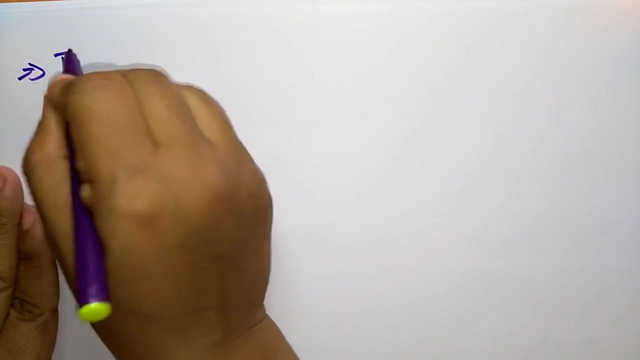 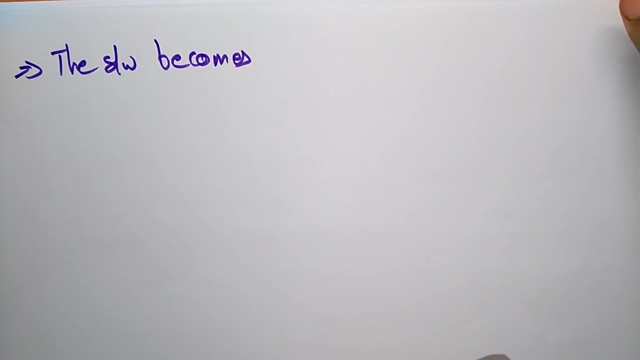 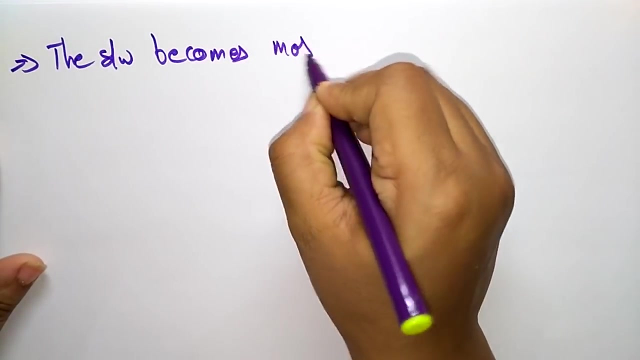 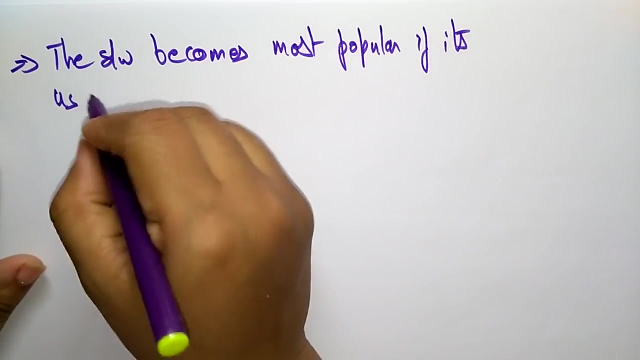 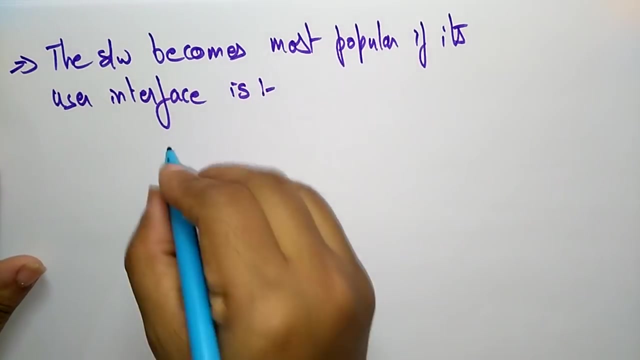 based to audio based, depending upon the hardware and the software combinations that you are using on the systems. okay, so the software becomes, the software becomes most popular when you can say that software becomes more popular, becomes most popular if its user interface is, if its user interface is attractive, simple to use. 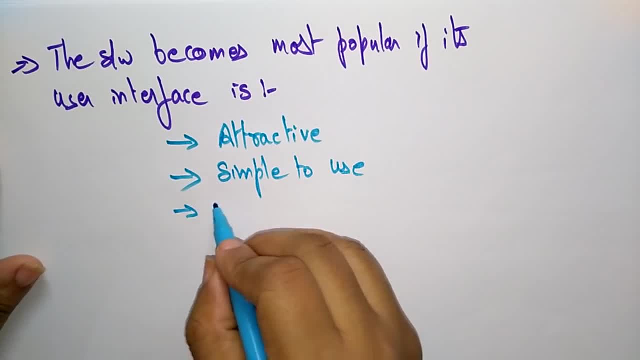 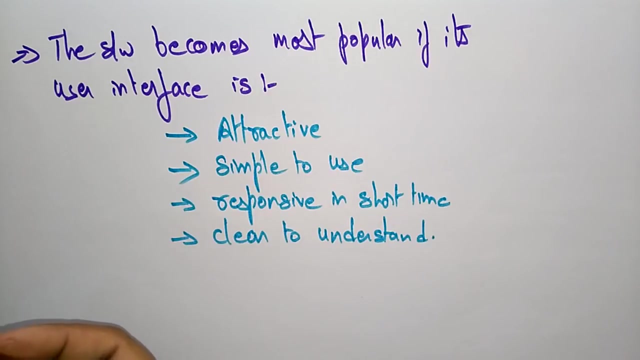 responsive in short time. responsive in short time and clear to understand. clear to understand, then only we can say that software becomes most popular. so if you take any mobile phone, okay, in your mobile phone you are installed some apps means some software you install. so when you it. 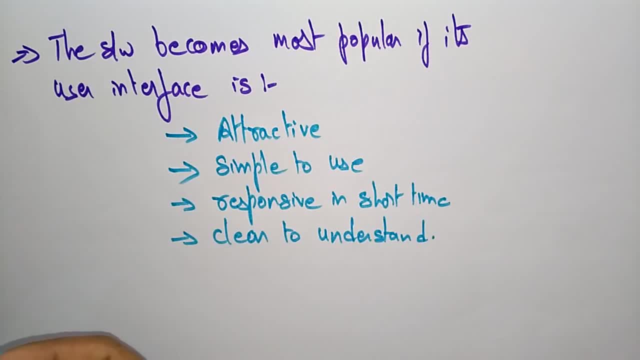 becomes more popular, When that app becomes most popular, when that app is more attractive. So if you are going to access that app, that software which is consisting of some user interface, So by seeing that app- suppose it is somewhat colorful and somewhat friendly-